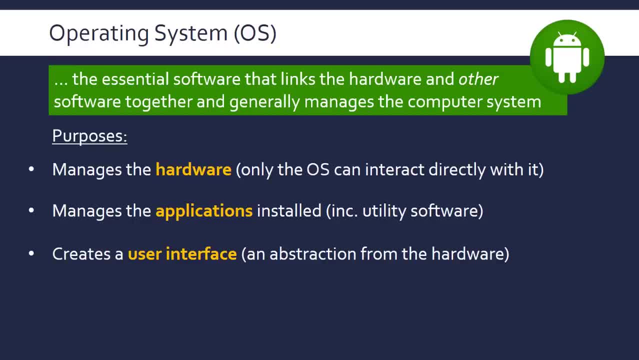 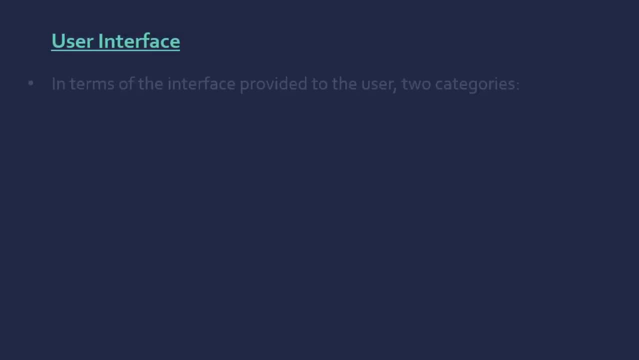 and, to put this in technical terms, you're basically abstracting from the hardware. and again, this is to do with kind of security, basically because the operating system is sitting as a bridge between the other software and the hardware. It's providing the security layer, this abstraction from the hardware. Just to expand on these a little bit more, then, First of all, the user interface. there are two main categories. First, we have a command line interface, CLI, and this is just a shell that responds to text commands, as you may have used or would have definitely seen. And then, of course, you've got your graphic user interface. 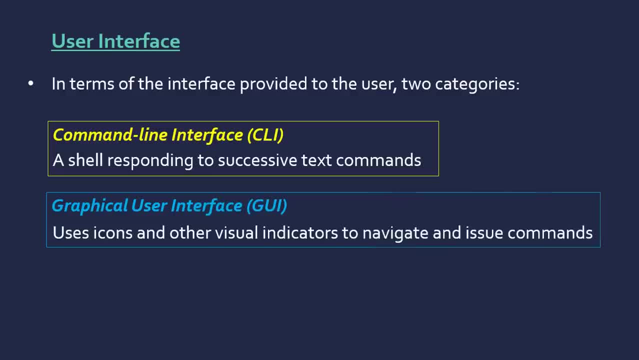 This is just icons and other indicators and menus and so on. So all major operating systems have this, but they have a command line interface as well. So in terms of evaluation, it's quite obvious why a graphical user interface is better. It's much easier in most cases. but in terms of doing a very specific instruction, people like to use the command line because it's much more direct. You can get it to do one thing without having to navigate loads of menus and so on, and therefore it's much more compact. You can chain your commands to do several things as opposed to just one thing. 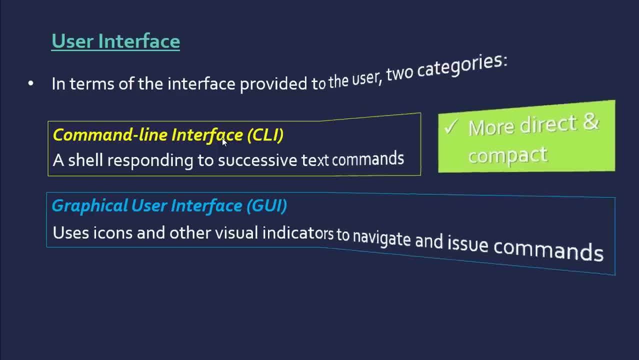 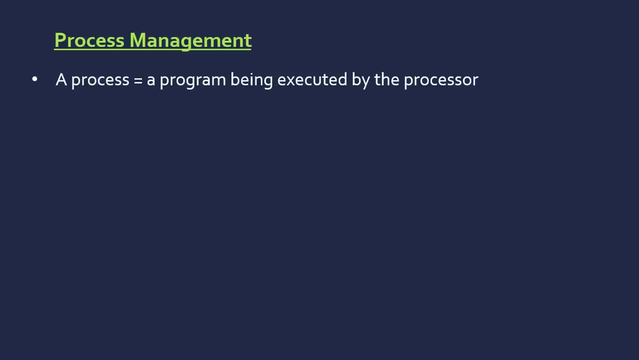 Moving on to a harder aspect, we've got process management, which is all about the operating system and the processor. So in this context, a process is a program being executed by the processor, So it's almost like what instructions are currently being executed by the processor. 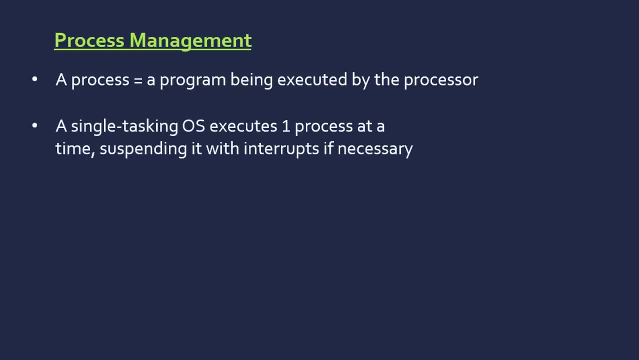 And just for comparison, really, because no operating systems are like this anymore. a single tasking operating system executes one process at a time, suspending it with interrupts if necessary. So basically, it executes process one, then process two, And an interrupt is basically a way of stopping what the processor is doing because something 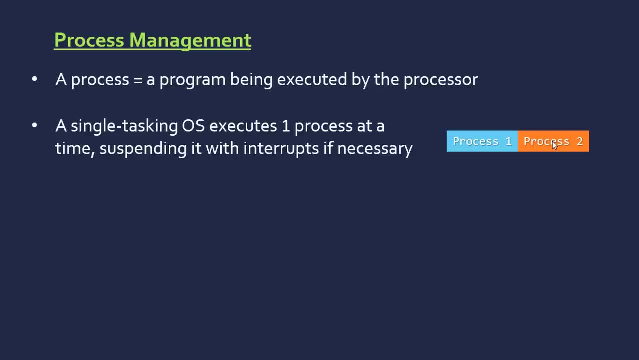 more important has come up. So, for example, the highest, the most serious interrupt would be: if you turn your computer off, It's got to suddenly save, or try and save, all your stuff, try and prevent data being lost. So it's got to immediately interrupt what it's. 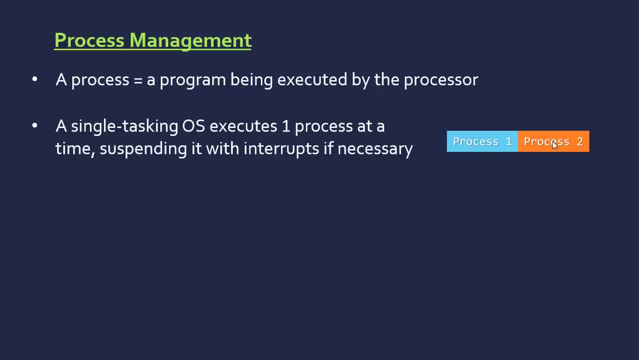 doing and run the interrupt code instead. But basically the whole idea of process management is a process is going to do one thing at one time. Even a multi-core processor- each core can only do one thing at one time. So it's all about maximizing the worth of each process. So some processes are more important. 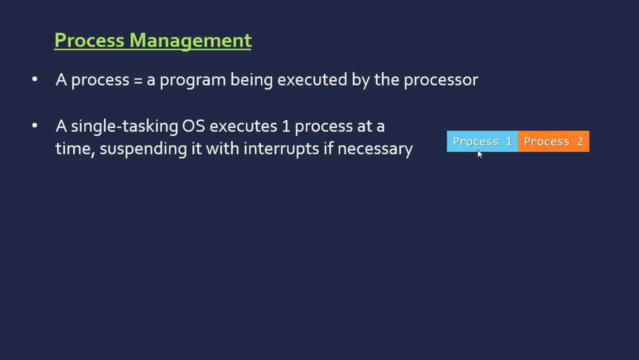 than others. So interrupts are more important than just general processes, general programs. So I said that's for comparison. Really, we're talking about multi-tasking operating systems which, again because of the limitations of hardware, execute one process at a time, but they allow multiple applications to run at the same time just by switching between processes. 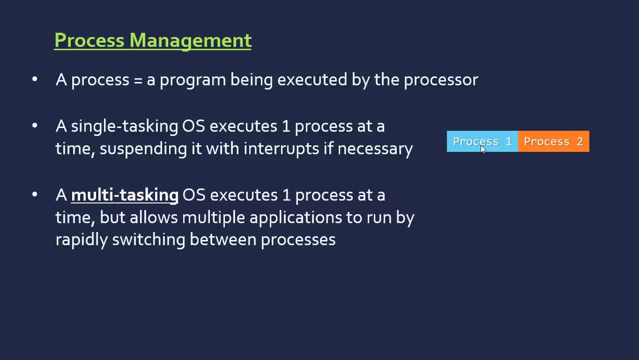 So in a single tasking OS, basically this represents one program. So you're running- I don't know- instruction on one program And then you terminate it, And then you terminate it and run another program, So you don't have programs running. 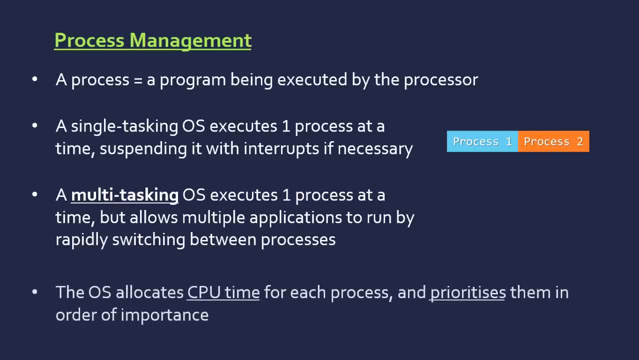 in the background. So the two things the OS does in this context is to allocate CPU time for each process, So the amount of time the CPU spends in one block for this process, because it's splitting up in a multi-tasking OS and also prioritizes them based on their importance So they can. 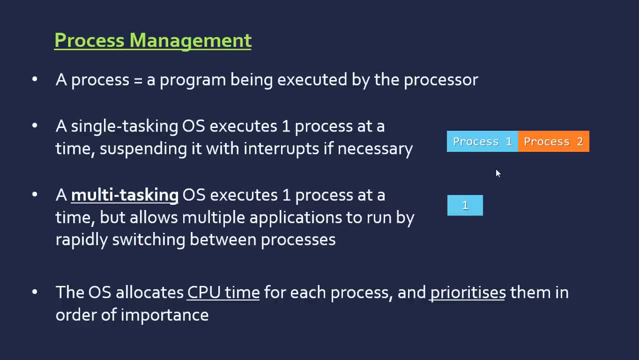 be allocated different CPU times based on their importance. So say: process one is given five clock cycles just arbitrarily and process two is given eight. Once it's finished with the eight for process two, it goes back to process one and then say: we've got an interrupt. 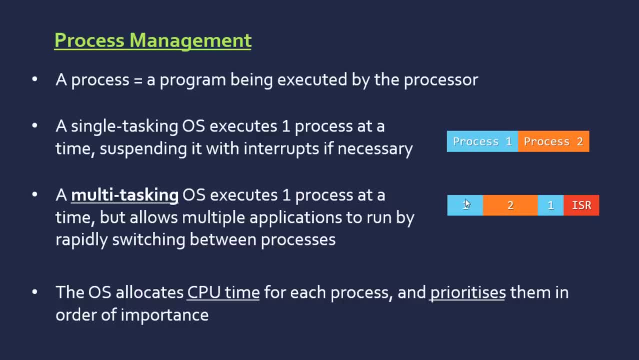 So say something's happened which requires immediate attention. we can see we've interrupted the CPU time and then it will finish off what's left over. So basically, a multi-tasking OS is juggling loads of different processes and it appears that they're running in the background, even though they're only ever being executed once. 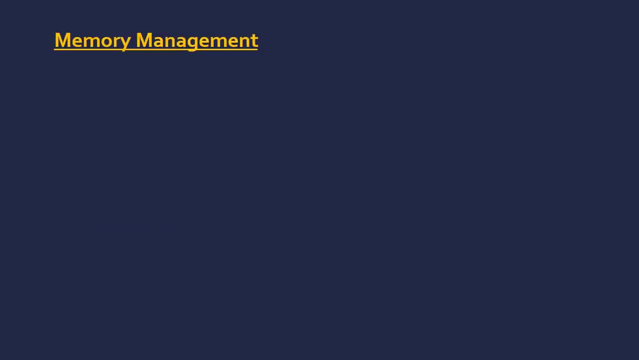 at a time. Some other management is also about allocation of resources and making that as efficient as possible, and this is all about memory space. So, as you may or may not know, when you open a program it needs to be loaded from the secondary storage like a hard drive into the RAM. 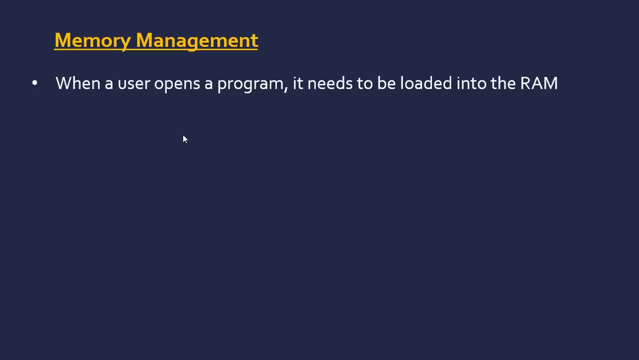 The RAM is much faster and is directly connected to the processor. so when you have a program and it's open and it's about to be executed, it needs to be copied into the RAM And, generally speaking, the memory system is what allocates and manages RAM space and so 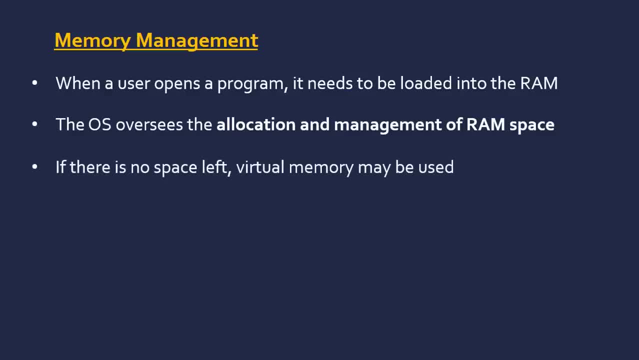 this process, So falling under this, if you say run out of memory because you've got too many programs open, It may. It may enact something called virtual memory, where it basically partitions a bit of a hard drive to act as if it's part of the RAM, so it extends the capacity, even though the hard 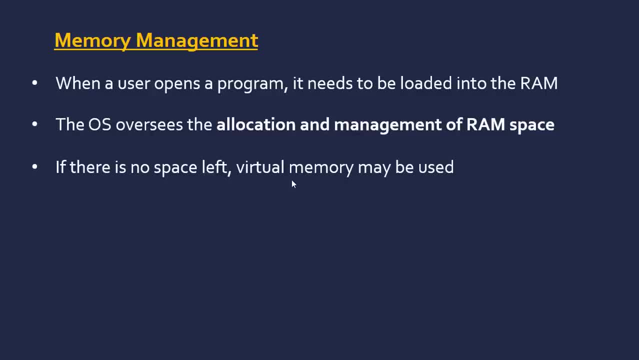 drive is much slower And there's a separate video on virtual memory, but you may not need to know about it for your course. By the way, just before I forget, the operating system itself has to be copied into RAM to be used. So when you turn your computer on, there needs to be a program to load the OS into RAM. so 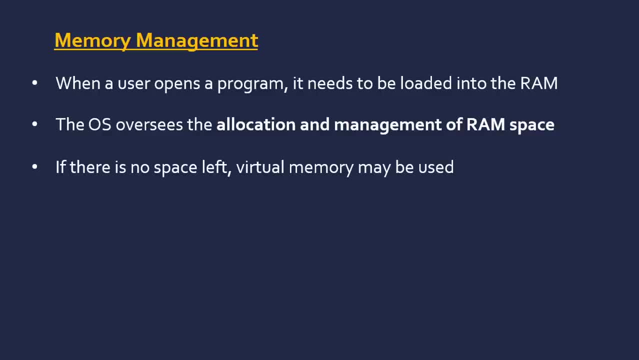 it can then do the rest of the process, and this is called a bootloader. It's a small program that may be stored on ROM on your motherboard, And its job is just to copy across the OS data from the hard drive onto the RAM, so that. 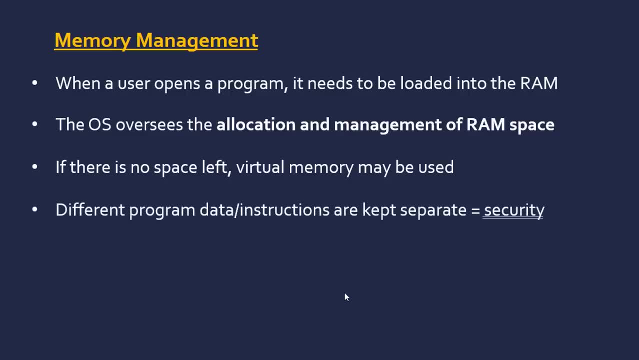 the computer can actually start up using the operating system. And finally, it's important that different data and instructions for different programs are kept separately in the memory and it needs to be clear which part of memory is for which. So this block is for program A and this block is for program B. 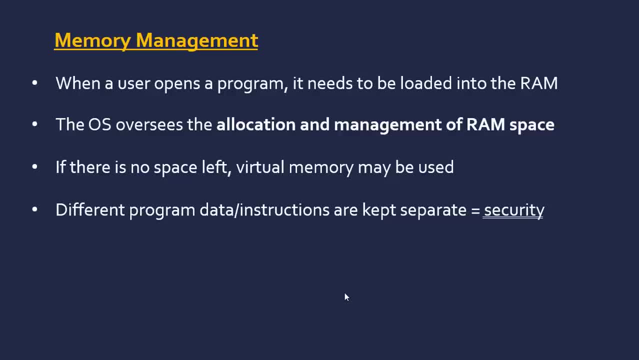 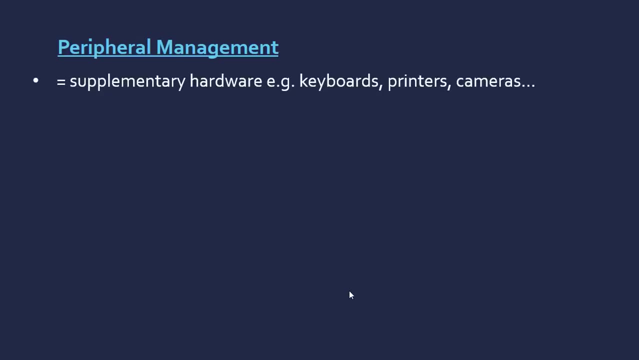 They can't access each other because that's a security weakness, obviously, and that's often where a flaw comes in To hardware, where different programs can access data where they shouldn't be able to. Moving on to look at peripheral management. So a peripheral device is just some supplementary hardware device like keyboard, printers, cameras. 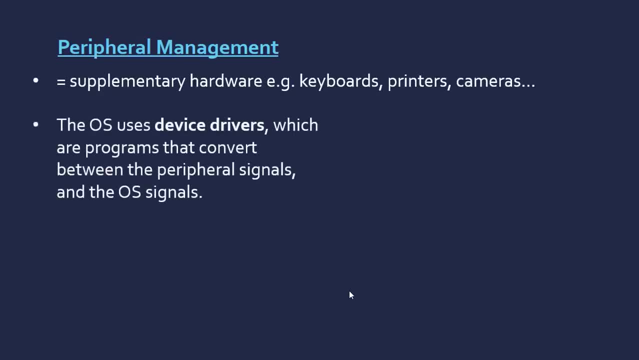 and so on. So I mentioned it right at the start of the video. but device drivers fall under the system software category and the only system that uses these, which basically are programs that convert between different signals used by each peripheral device and the OS. So basically it needs to be a conversion between: 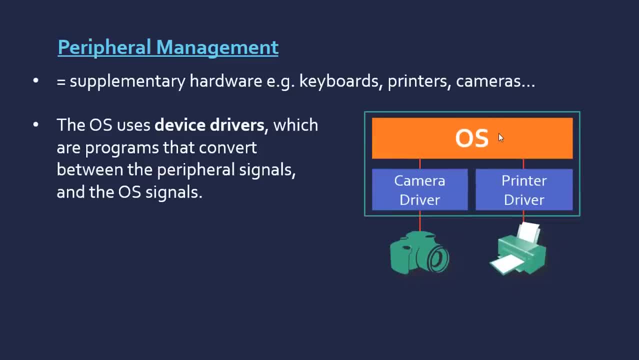 Whatever the camera is using and whether the OS is designed to use, and so on. So a Sony camera may produce different signals to a Canon camera and the driver specific to the device has to convert to the generic input the OS is expecting. So the term interface, which can be used both in the literal sense like an interface, you 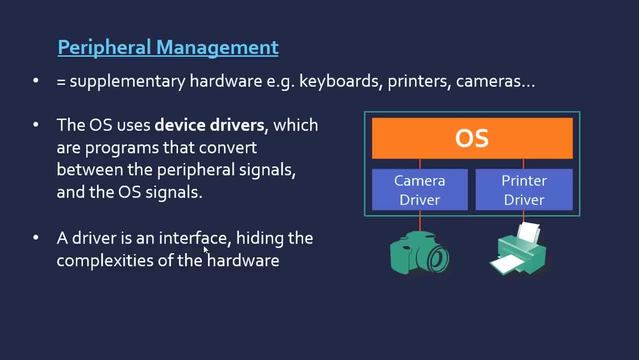 can interact with, or just a abstracted sense. A driver is an interface. it's hiding complexities of the hardware. The OS doesn't need to worry about being designed to work with every device on the world. It can use the driver just to convert to one type of signal. 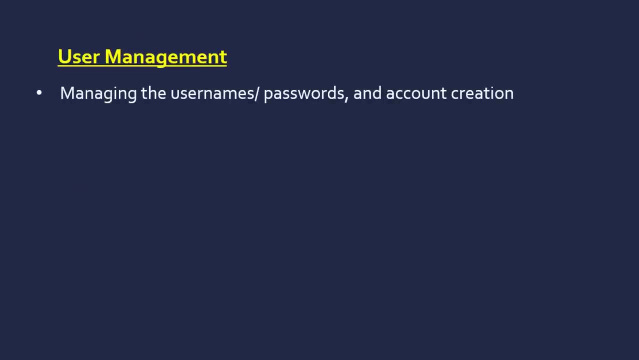 So just two more points you need to know about. So user management is an aspect all about maintaining and allowing creation of user accounts, and so the operating system needs to manage username, passwords and so on, And it's worth bearing in mind that not all operating systems actually allow multiple.